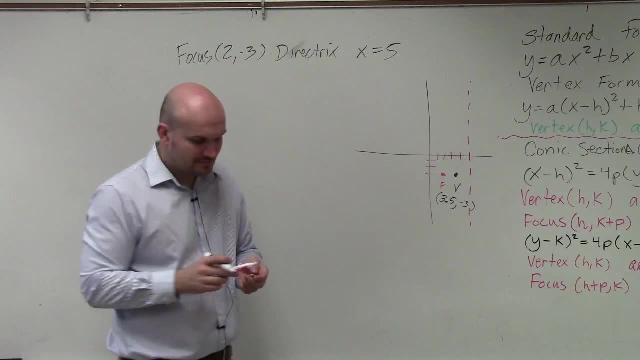 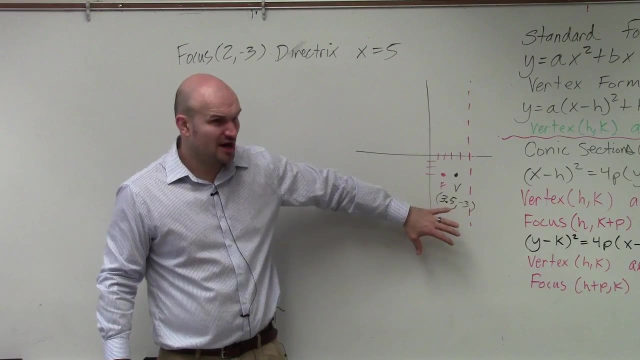 The same thing happens. The axis of symmetry is going up. Now the other thing: remember a parabola opens up towards its focus. So am I opening up or down? No, and I'm not opening to the right, so I'm opening to the left. 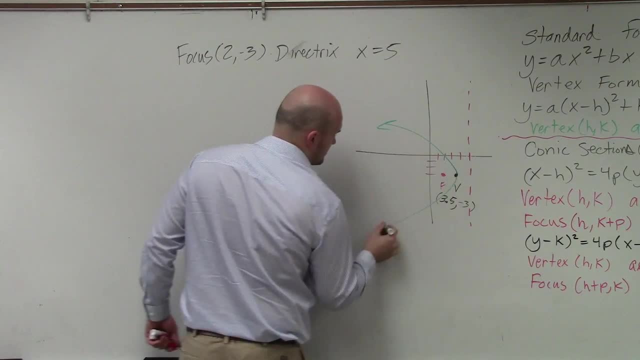 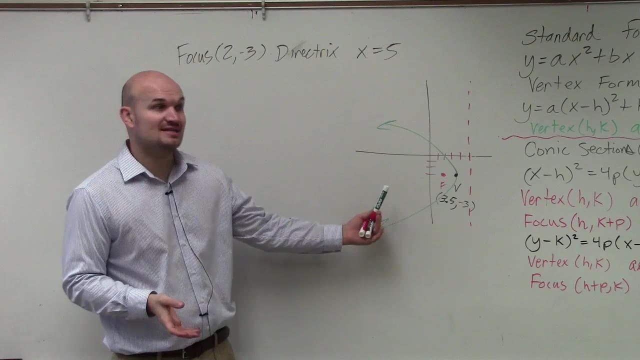 So my graph looks something like this, Just something like that. The only thing I notice is: hey, okay, now this graph is opening up horizontal, so therefore x is not going to be squared, because I'm familiar with the parabola, where x is squared right. 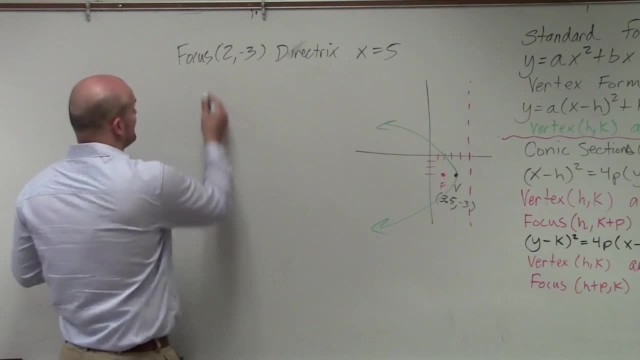 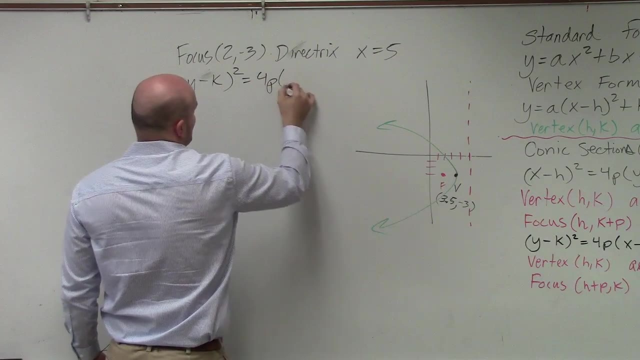 So therefore y. So y has to be squared. so we look at our formula that we used for that and we have y equals- I'm sorry, y minus k. squared equals 4p times x minus h. Now we identified our vertex. 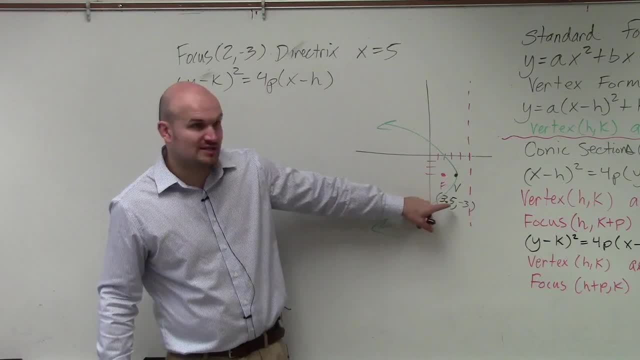 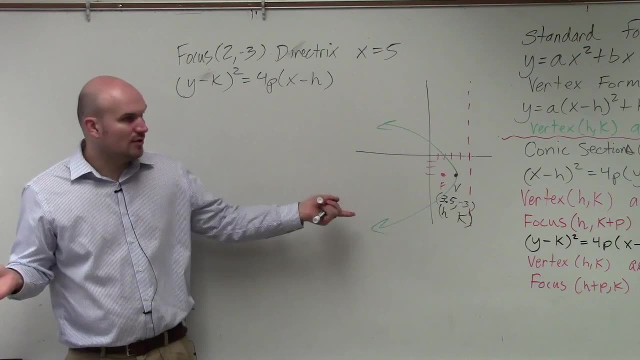 We had to find the coordinate point for the vertex. So the coordinate point for my vertex, this is my h and that's my k. The last problem: the vertex was at correct. So now we have a vertex at h and k. 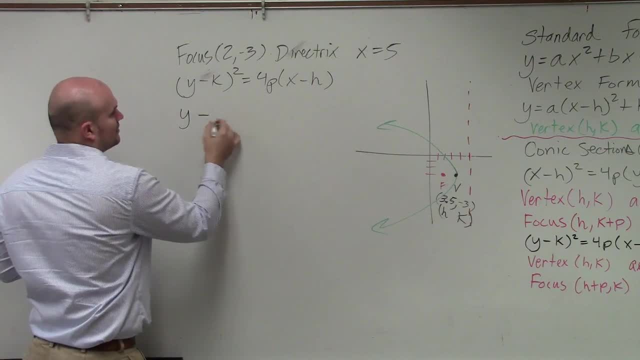 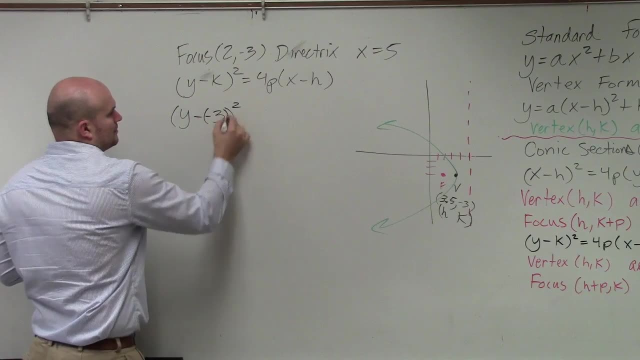 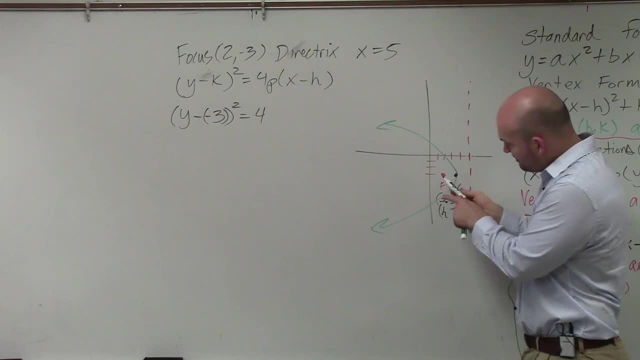 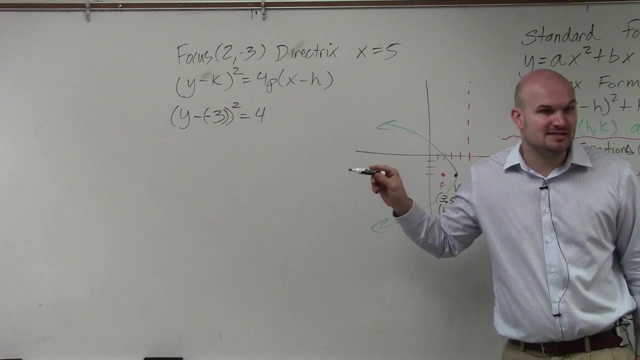 Now p is important. We know that the distance from my vertex to my focus was 1.5. But to go from my vertex to my focus, I'm going to the left. So is p going to be positive or negative, Negative? 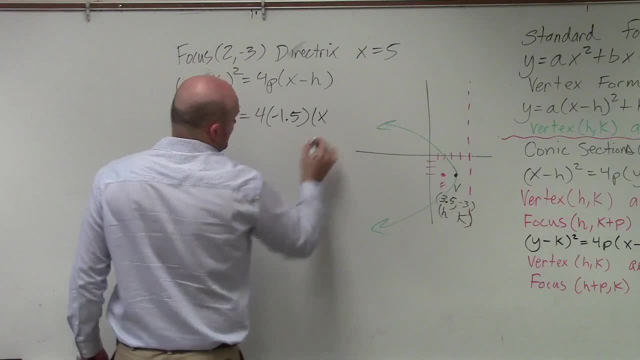 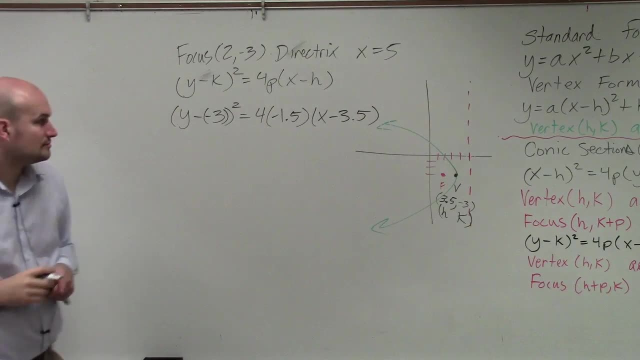 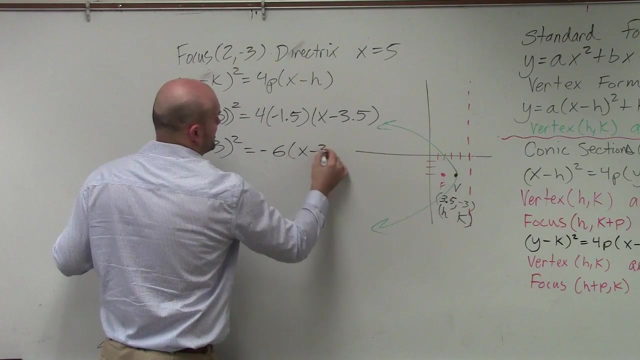 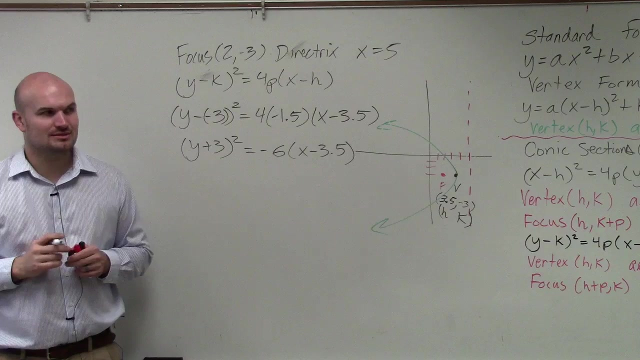 And then that's going to be x minus h, So it's minus 3.5.. So now we just simplify: y plus 3 squared equals negative 6x minus 3.5.. Any questions? Okay, The main important thing, guys, I'm telling you if you guys can get. 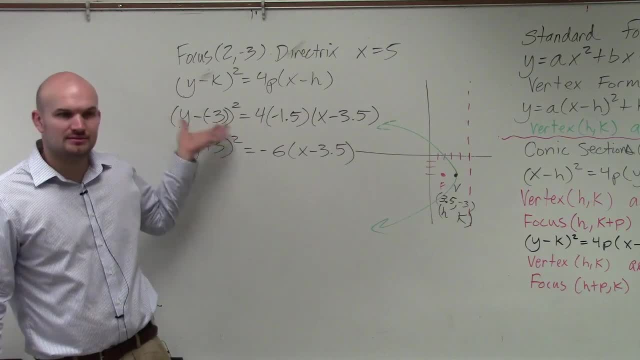 this stuff. right then, all you're doing is just throwing in the numbers in there in the formulas. But the main important thing is knowing what the parabola looks like. and then